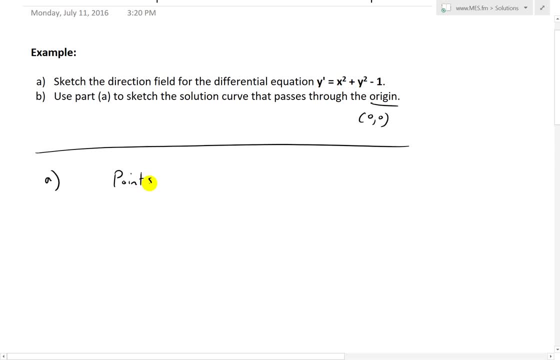 we basically could write this as so, if you were to get a table, either a table, you just either do it manually or use Excel calculator or an online calculator. I'll pull out an online calculator soon. So the y prime, this is the slope. So, for example, the point 00,. this slope is going to be equal to, well, zero squared plus zero minus one. that equals to negative one. and then the point 01, for 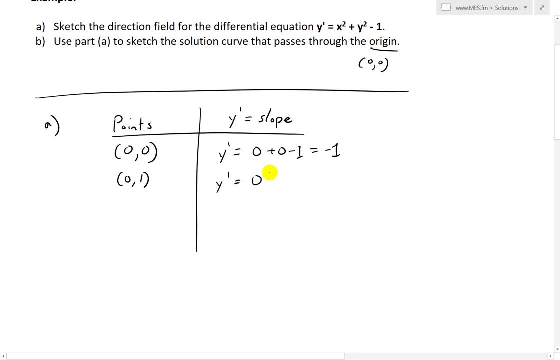 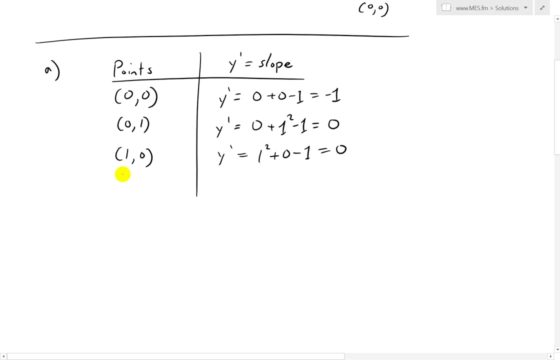 example, this is what crime equals to zero, and this is zero squared plus one squared One squared is just one minus one. this again, this just goes to zero, And similarly one zero. This will be y prime. this equals to one squared plus zero minus one equals zero again. let's let's look at a more complex one zero two, So this one that this point will have a. 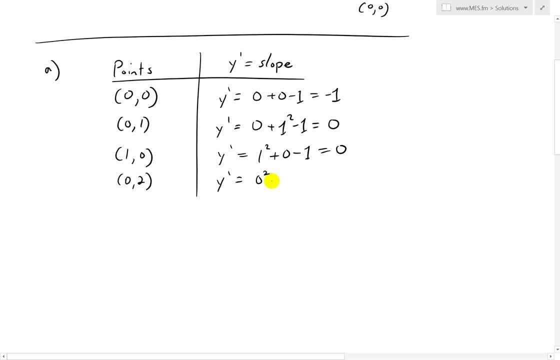 up again. 0 is the X, and then the Y is 2, 2 squared minus 1, so this is 4 minus 1. that equals to 3, so it's a steeper slope. and again, basically, you do this for a bunch of points, however many you want, which is actually better, so you can dot. 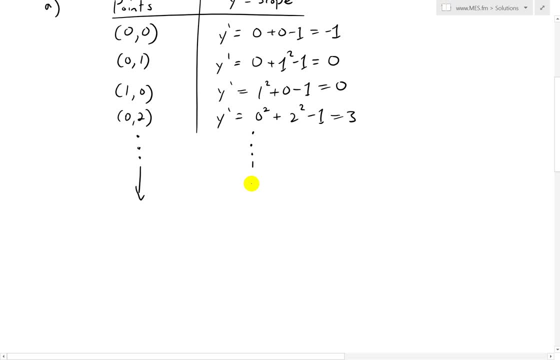 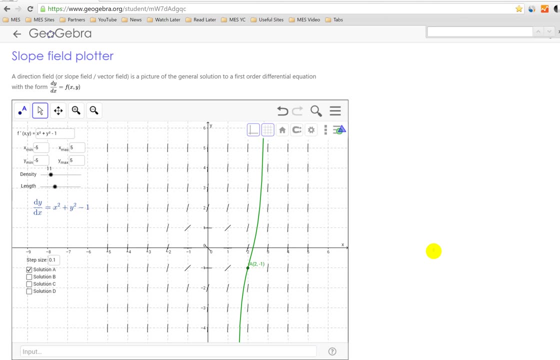 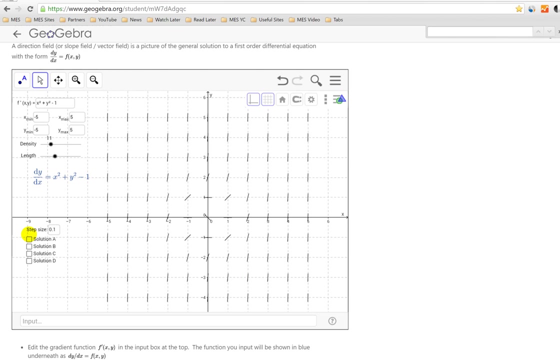 dot dot, go down and then solve the slopes for each single one. keep going as many as you need. and here I've just. this is just a random direction field or slope field plotter generator that it's pretty useful. it's again. I went over this one in my last video. basically, if we were to look at this graphs when you 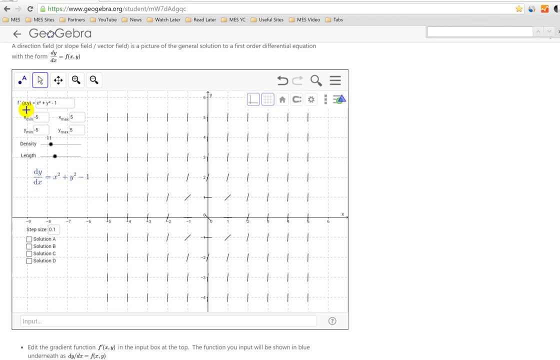 plug it in in this case is our differential equation: f of f, prime of x, y is equal to x squared plus y squared minus 1. or again, dy over dx equals x squared plus y squared minus 1. so that's the difference between the two and the 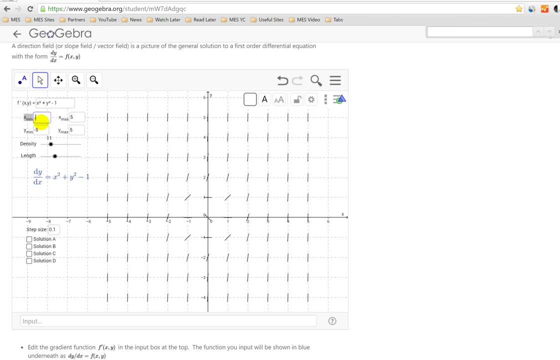 y squared minus 1. so that's just our equation and I'm going to change these up like that just to get with. my calculus book has the coordinates from 2 to etc. so something like this. and again, those are the slopes of at each and one. 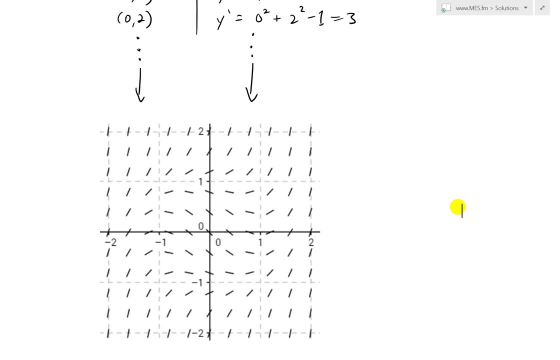 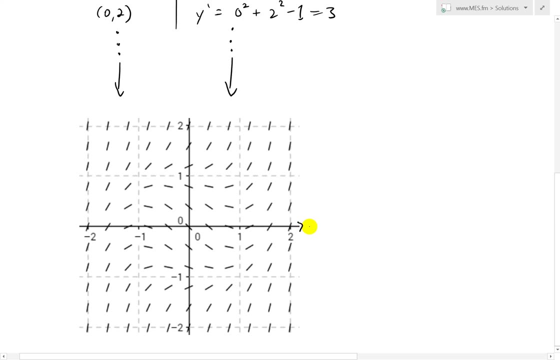 of these points and I'll- I've copied it over here, yes. so here I've copied that same plot here, zoomed in and then, as you can see here, we have this extends and we'll have the y and x-axis. so these are all the directional fields, as you can see here. 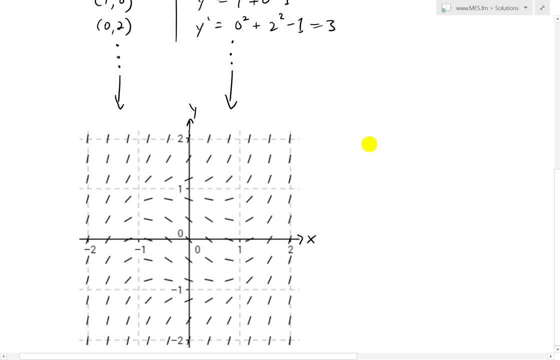 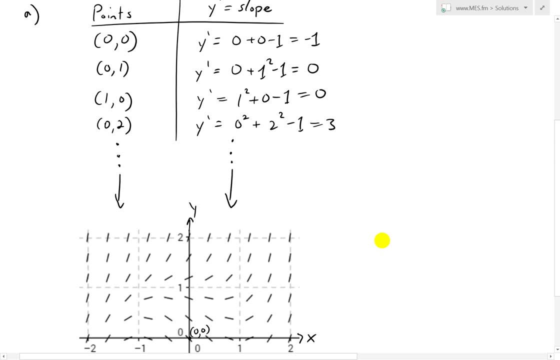 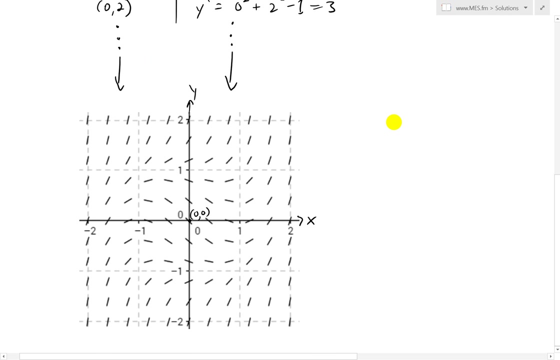 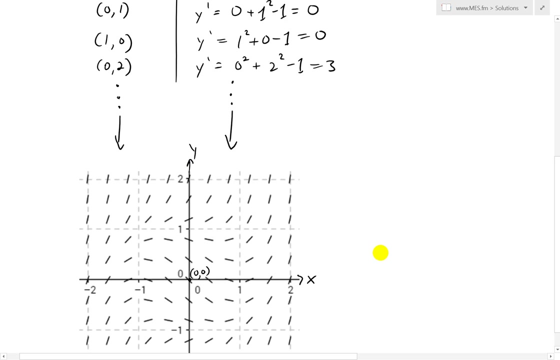 at the point zero, zero. it's a negative 1 slope, which is again that's our negative 1 slope. this is our zero, zero point right here, and then when we go up to that is basically that is at the point 0, and then one actually doesn't have 1. here is in between. yeah, actually had that one in general. 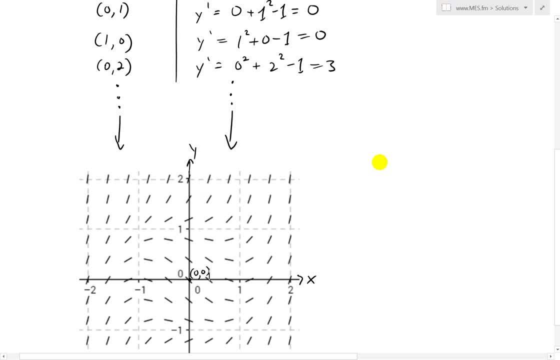 one there, but let's look at the other one, 0, 2, which is yes. so the 0, 2 point that's over here, as you see, that's very steep as compared to this negative one. so it's, yeah, that's pretty much represents it, yes, so now the next step. 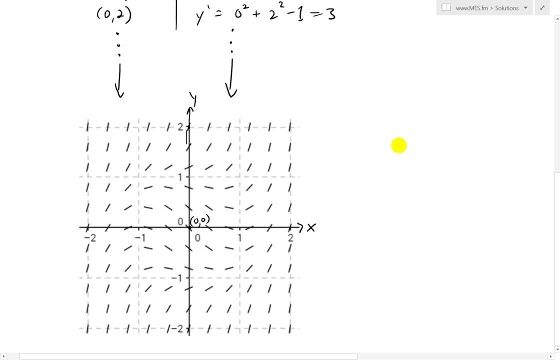 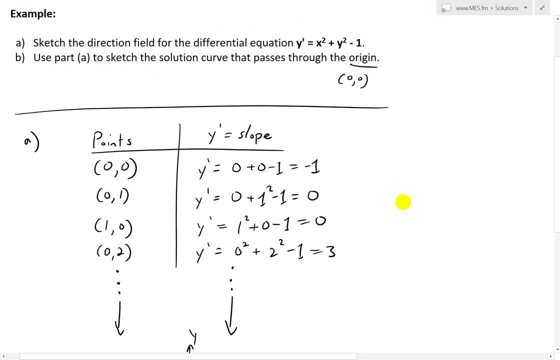 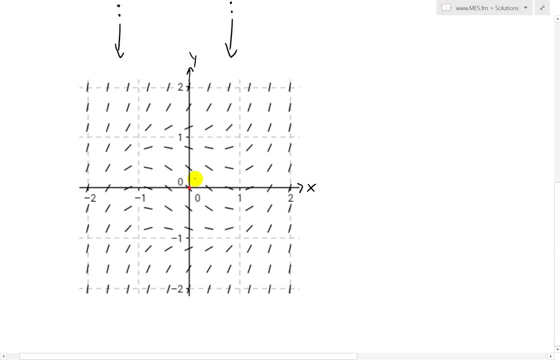 is is part B, because basically this is our direction field generated. you can do this manually. I just got that random calculator online. so part B states: use part A to sketch a solution curve that passes through the origin, so this origin. I'll draw this actually in red. so this is 0: 0. so if you were to draw a, 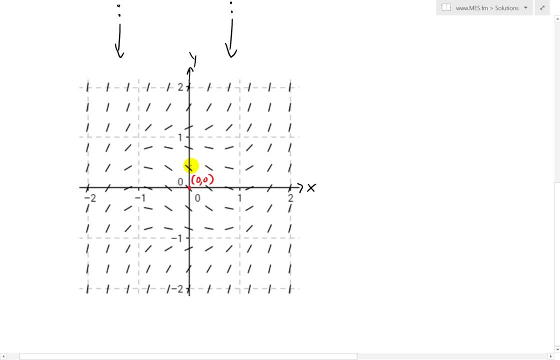 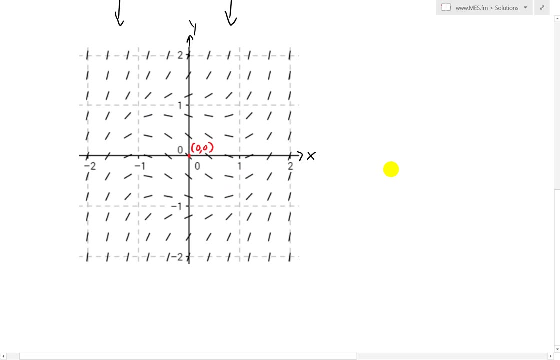 solution curve that goes through here and again these direction fields or the end. these are pretty much small line segments that roughly estimate the solution curves. so at this point if we were to go to the right, we're gonna have to go downwards, like this, because the slope is negative, and then, as you can, 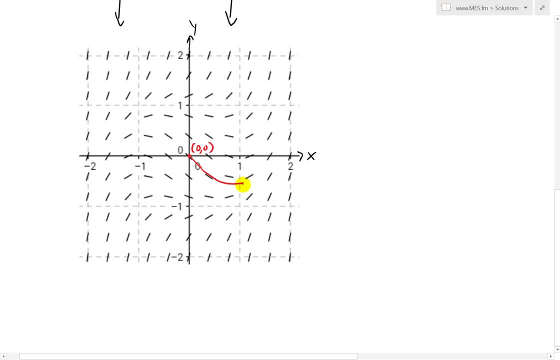 see the slope is becoming uh positive, so goes to zero than positive. so we're going up and, as you can see, we are going up like that- I'll draw this a bit neater, or something like that- and then, on the left side again, this is slope is going up like that and it's. 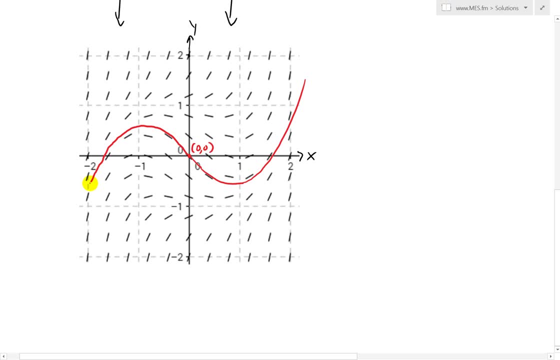 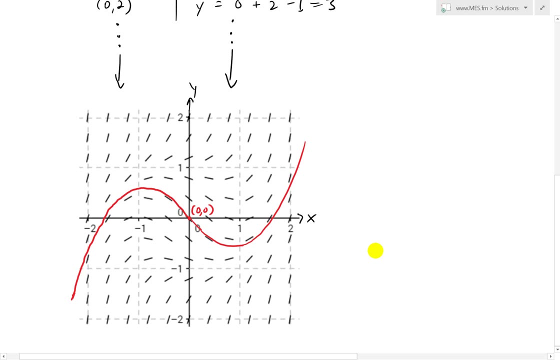 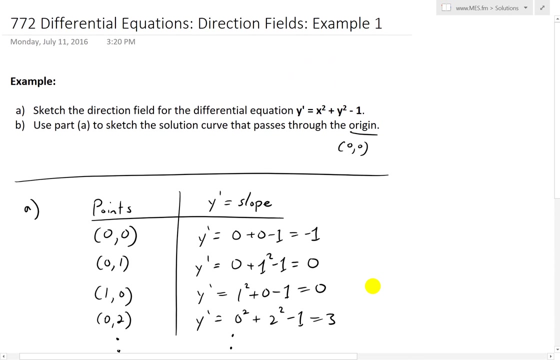 breaking down and then, because we're gonna just have to be parallel to the lines, roughly to the slope, so go something like that and this is. yeah, this is pretty much how our solution curves look like, and we did not even have to find the solution explicitly, we just roughly estimate that the graph would look like.